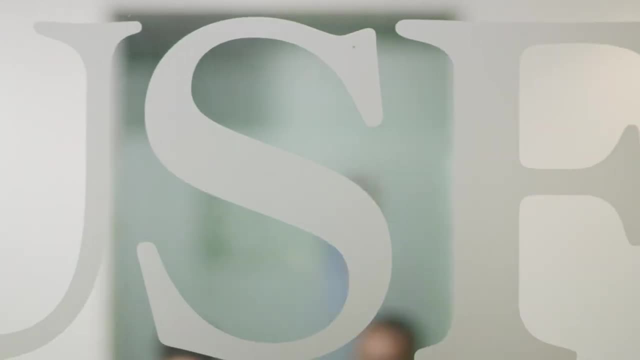 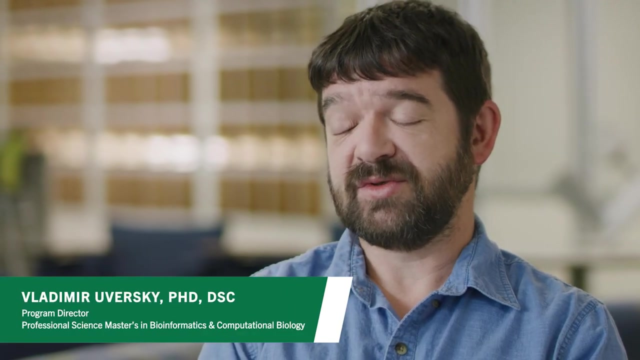 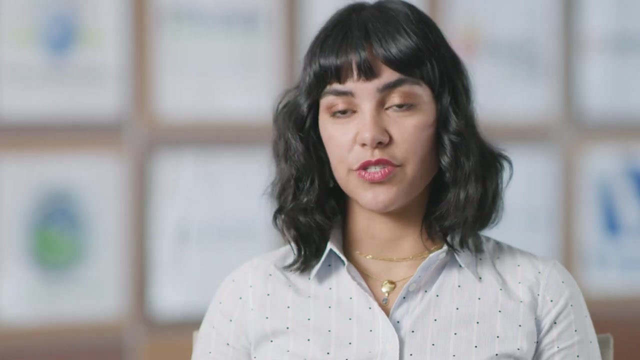 Bioinformatics program at USF is really very good. So we are very friendly to students. We accept students with different backgrounds. This program has been really useful in that it allows for great collaboration between students, researchers, research institutions and hospitals, And then USF really offers a supportive environment for students. I was 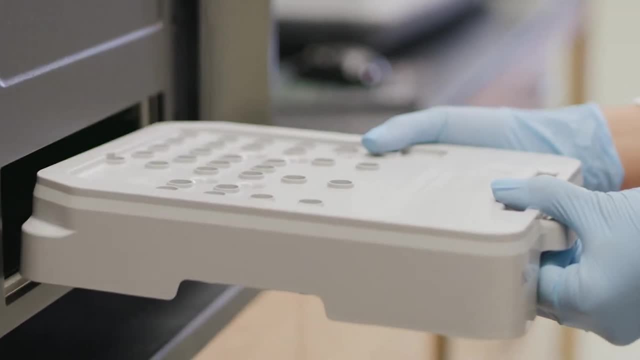 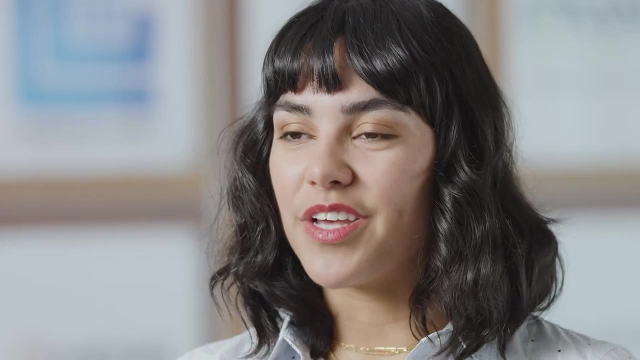 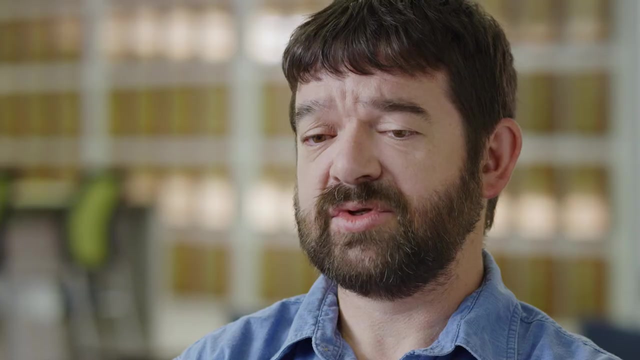 given funding to present my research around the US and abroad and I really appreciated that level of direct interaction between professors, conferences, students. So the collaborative environment was a big draw. Program started more than 10 years ago. It was one of the first professional master's. 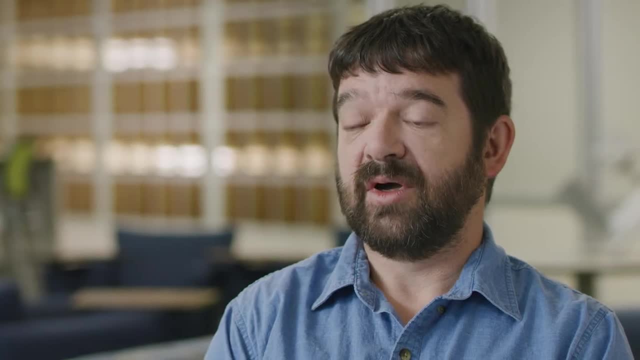 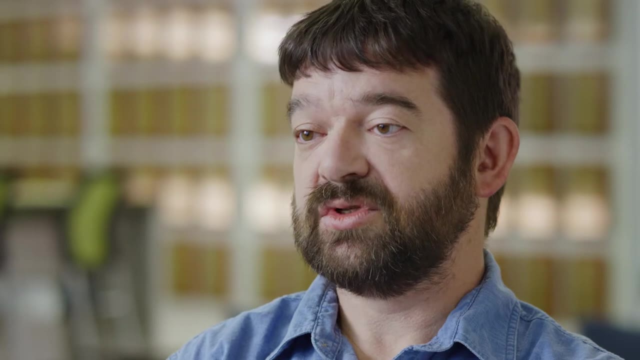 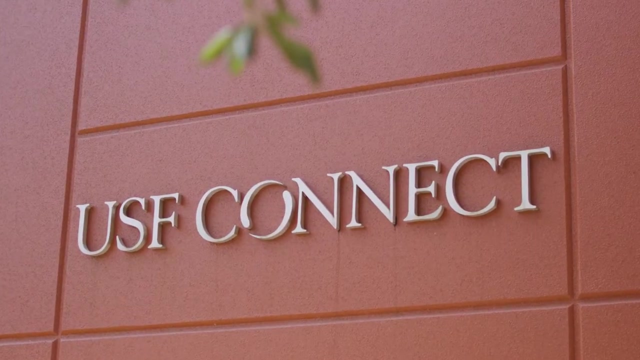 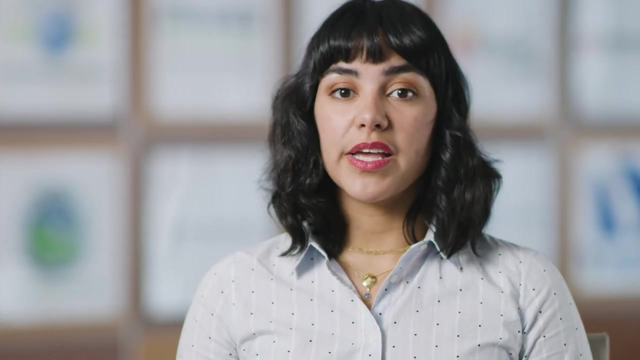 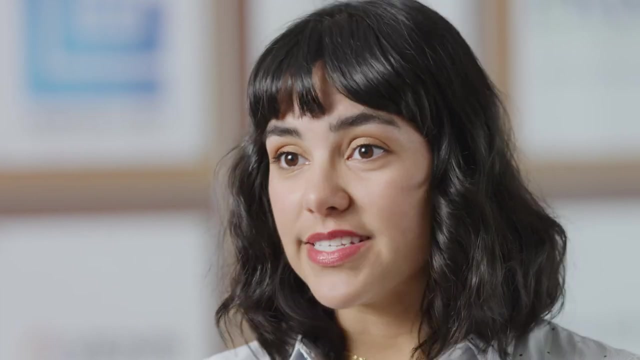 program in Florida Focused on providing pretty good background on bioinformatics given hands-on experience to students. So students in our program are participating in real scientific projects. I have done research focused on everything from immunology to cancer genomics to public health. I was able to go to London and to Montreal in Canada, as well as San Antonio. 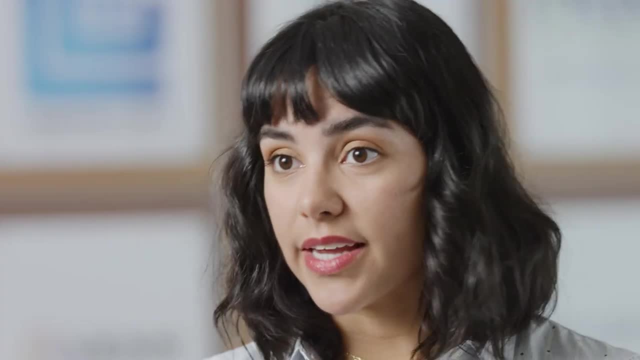 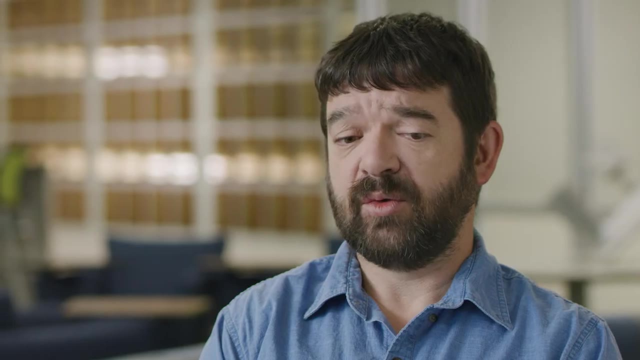 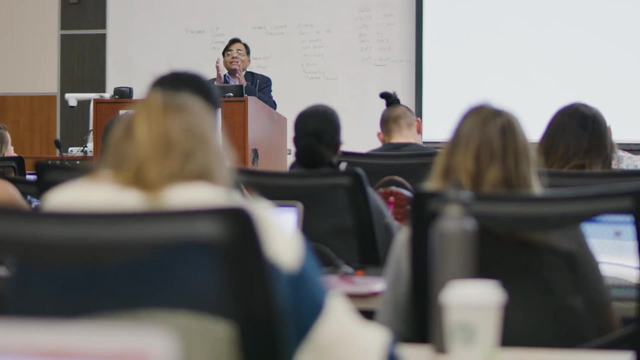 and San Francisco and present research. It was wonderful to be able to make connections in many conferences and speak to researchers around the world. Students from our program are typically deciding to go for next level of education, So we have students who are going for PhDs, we have students who are going for medical doctors and we have 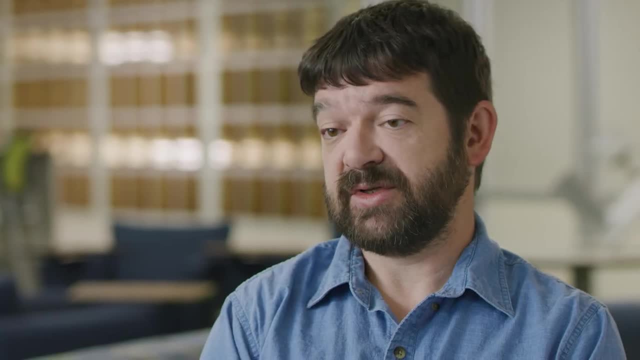 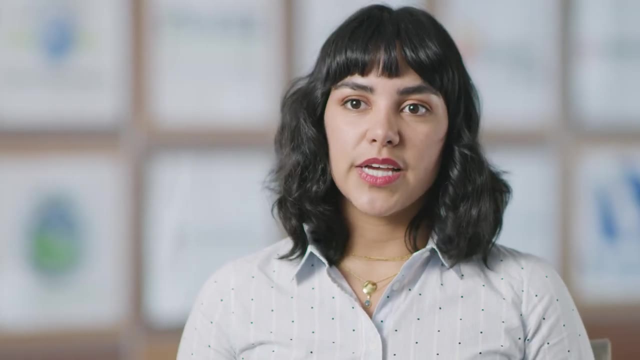 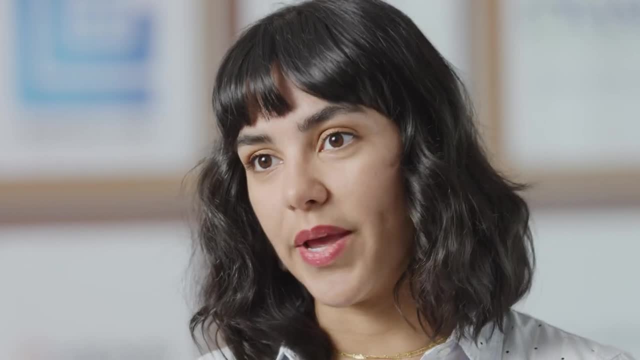 I'm going to be a PhD student at McGill University. I'm going to be a PhD student at McGill University in Montreal And it's a collaborative program with Kyoto University in Japan. We are giving students a very good background in research. We are providing them with very good knowledge of bioinformatics. So once again, we are good.